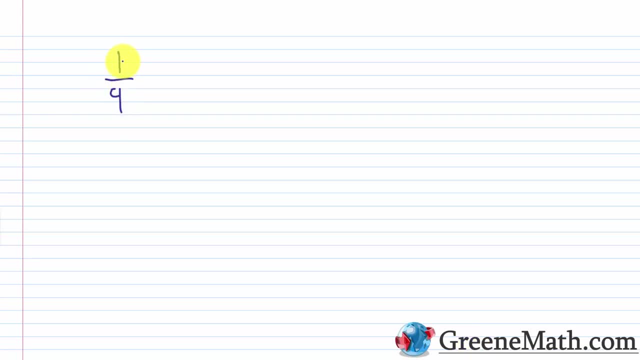 So something like the number 1, 4th. 1 is an integer, 4 is an integer, So you have the quotient of two integers. The denominator is not zero, So that's a rational number. Something like negative 7, 5ths, Something like 11, 14ths, Something like just the number 10,. 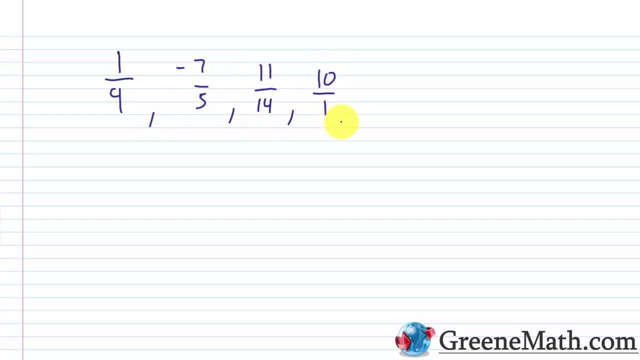 right. 10 could be 10 over 10.. Right, So all of these fit that description. The main thing to understand here is that we can't divide by zero, so we can't have zero in the denominator. Okay, so that's very important. 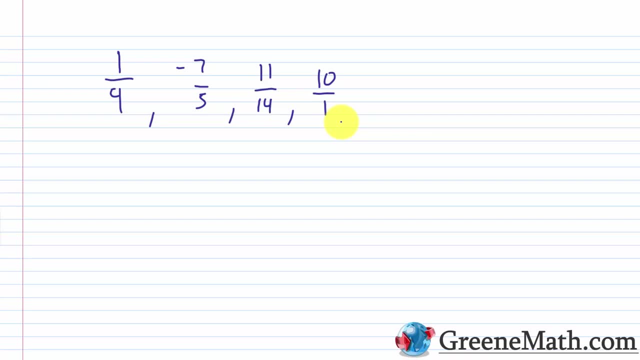 Now we think about these as rational numbers, but more practically we just call them fractions. So in algebra we have an algebraic fraction. This is known as a rational expression, And what this is is. this is the quotient of two polynomials where the denominator is not zero. 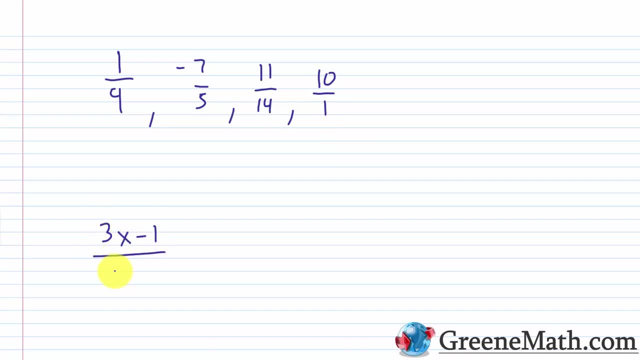 So something like 3x minus 1 over, let's say 5x squared plus 2. One polynomial over another. So that's a rational expression. As another example, let's say you had 2x squared plus 5x minus 1 over, let's say 3x to the 4th power plus x plus 7.. Okay, so you have a polynomial up here. 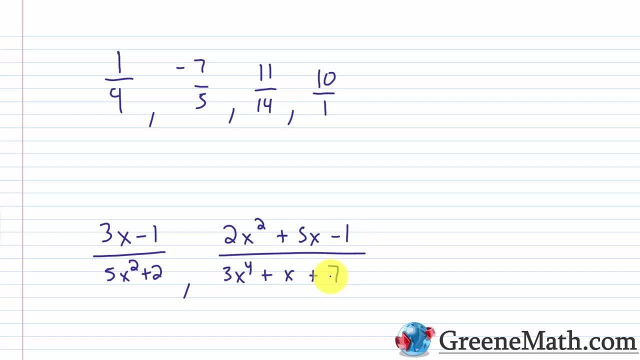 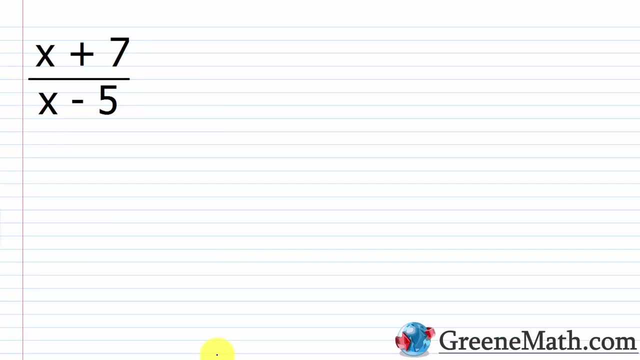 a polynomial down here. So one polynomial divided by another. Again, that gives us a rational expression. So essentially, when you start working with rational expressions, the first topic you come across is how to find the restricted values for a rational expression. Now this topic just basically deals with division by zero. We know that we're not allowed to divide. 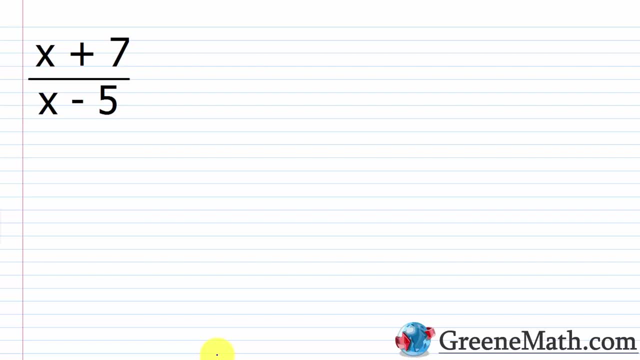 by zero. If we see something where we have division by zero, it's considered undefined. So something like 3 over zero. Let me make that three a little better. This is undefined. Okay, that would be your answer there In the case- and I know some of you will be confused and say no. 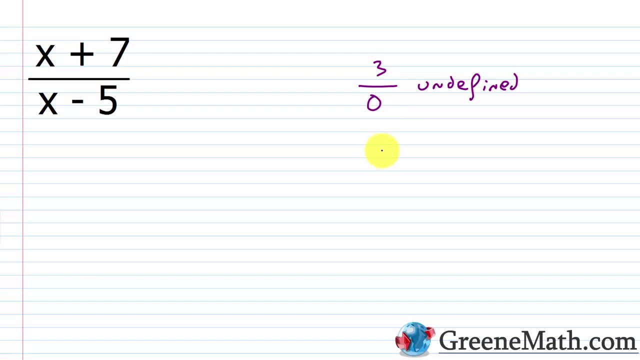 three over zero is zero. That's not right. right. When you divide zero by a non zero number, you get zero. So zero divided by three would be zero. Okay, you can divide zero by anything you want, except zero, you get zero. But if you try to divide by zero, it is undefined Okay. So if I had 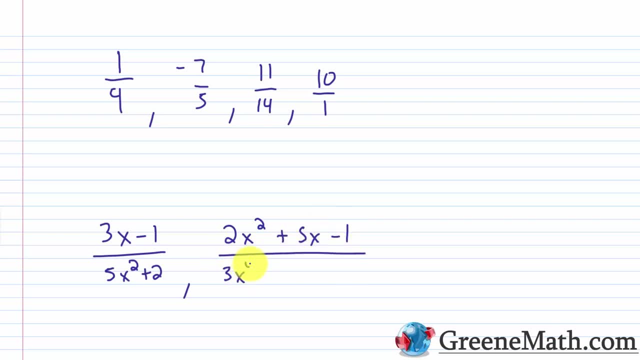 minus 1 over, let's say 3x to the fourth power, plus x plus 7, okay, So you have a polynomial up here, a polynomial down here, So one polynomial divided by another. again, that gives us a rational expression. So, essentially, when you start working with 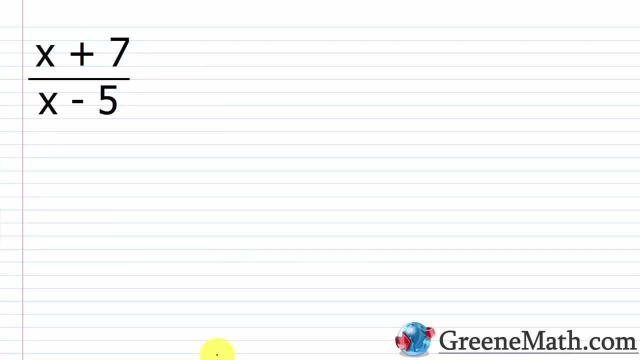 rational expressions. the first topic you come across is how to find the restricted values for a rational expression. Now, this topic just basically deals with division by 0. We know that we're not allowed to divide by 0. If we see something where we have division by 0,, 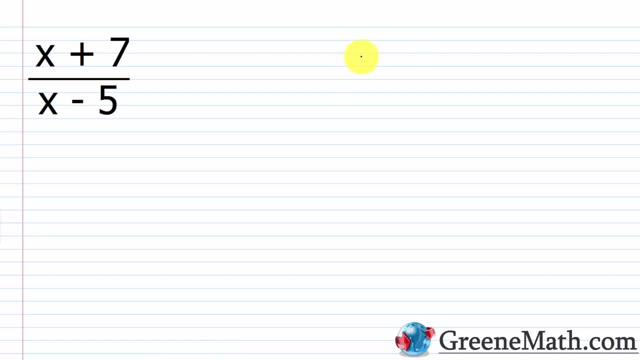 it's considered undefined. So something like 3 over 0, let me make that 3 a little better- this is undefined. okay, That would be your answer there In the case- and I know some of you will be confused and say no, 3 over 0 is 0,. 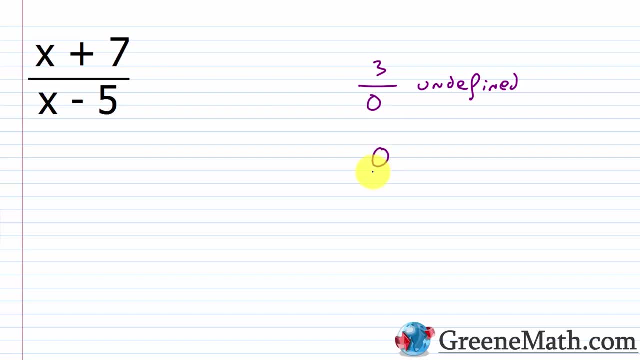 that's not right. right, When you divide 0 by a non-0 number, you get 0. So 0 divided by 3 would be 0,. okay, You can divide 0 by anything you want, except 0, you get 0. But if you try to divide by, 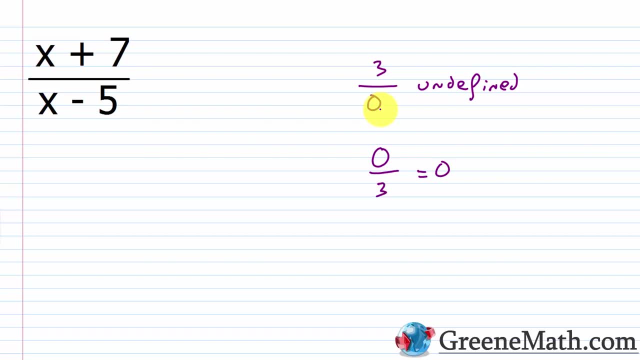 0,. it is undefined, Okay. So if I had a rational expression like x plus 7 over x minus 5, what would be my restricted value here? Well, it's anything that makes the denominator 0, okay. So if I look at my denominator, 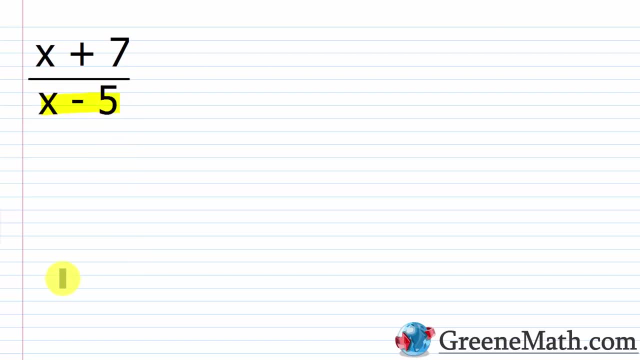 it is x minus 5.. So how do I find the value for x that makes this denominator 0?? All I need to do is set my denominator equal to 0, and just solve right. What am I doing? Something minus 5 gives me 0,. I'm going to solve for that. 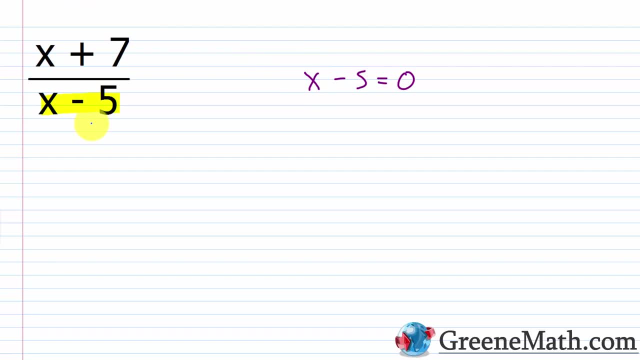 something so that I know what I can't plug in for x. It's just that simple, So very easy. we just add 5 to each side of the equation. this will cancel. we'll have: x is equal to 5, okay. 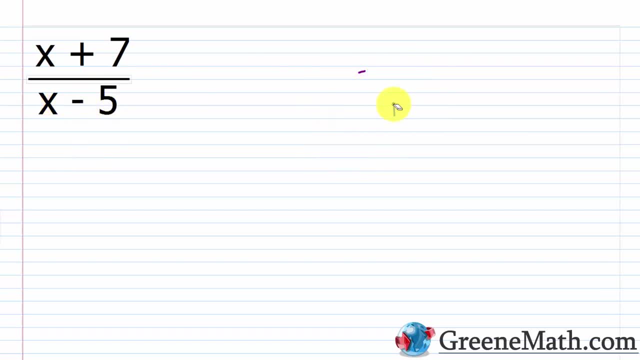 And you can easily see if I let x be equal to 5,, let's say that we let x be equal to 5, plug in a 5, here and here, so you would have 5 plus 7 in the numerator, which is 12, over the denominator would. 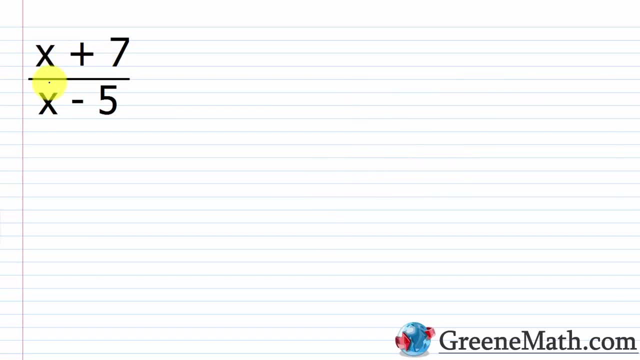 a rational expression like x plus 7 over x minus 5. what would be my restricted value here? well, it's anything that makes the denominator zero, okay, so if i look at my denominator, it is x minus 5. so how do i find the value for x that makes this denominator zero? all i need to do is set my 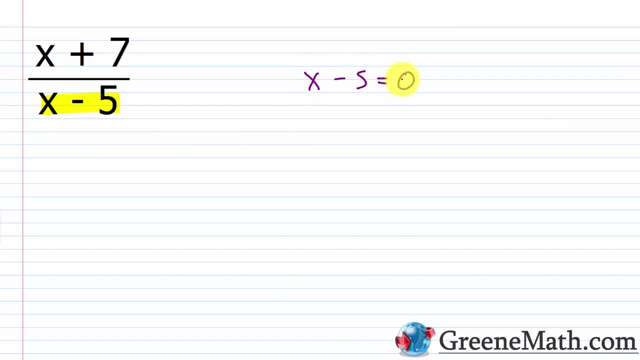 denominator equal to zero and just solve right. what am i doing? something? minus 5 gives me zero. i'm going to solve for that something, so that i know what i can't plug in for x. it's just that simple, so very easy. we just add 5 to each side of the equation. this will cancel. we'll have x is. 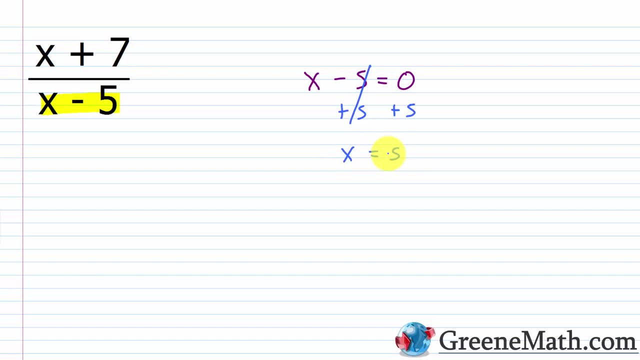 equal to 5. okay, and you can easily see if i let x be equal to 5, let's say that we let x be equal to 5 and i'm going to solve for that something, so that i know what i can't plug in for. 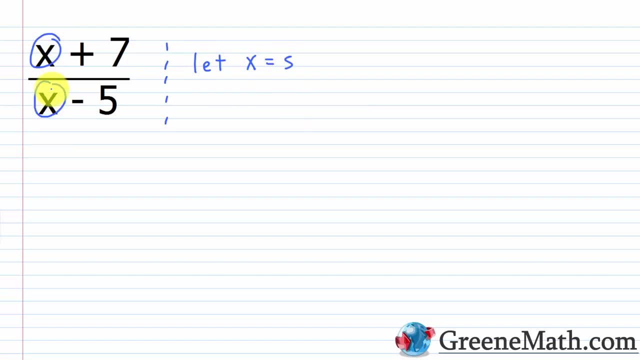 be equal to 5. plug in a 5 here and here, so you would have 5 plus 7 in the numerator, which is 12, over the denominator will be 5 minus 5, which is of course 0, and again this is undefined, and this is what we're trying to prevent. 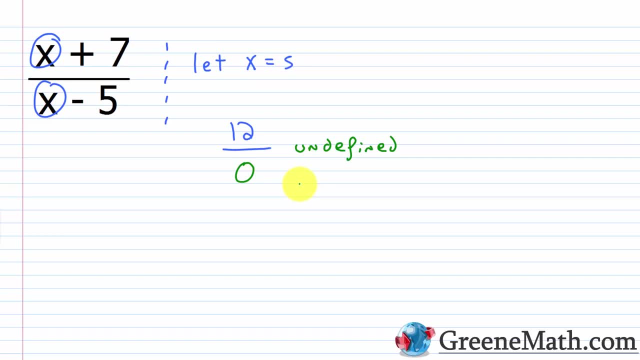 we don't want to end up with something that's undefined. so what we do when we have a rational expression is we find our restricted value, or our restricted values, depending on how complex your rational expression is. and we just put a little note here. we say that this is defined for everything except for X. when 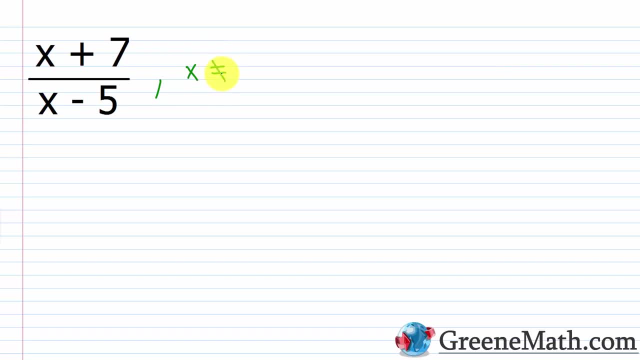 it's equal to 5. so we'll put X cannot be equal to, or X does not equal 5, okay, a fancier way to do this is to state the domain. okay, so the domain, in case you haven't seen anything with functions yet. we'll talk more about this later in the. 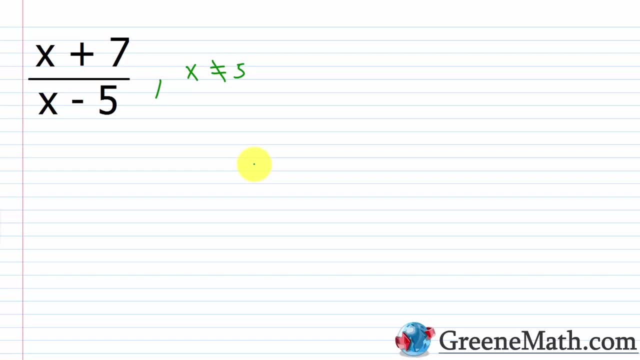 course, the domain is the set of allowable, unallowable, unallowable, unallowable, unallowable, unallowable, unallowable- X value. so what is allowed to be plugged in here for X? well, everything in terms of real numbers can be plugged in for X except for 5. so the domain, or again the 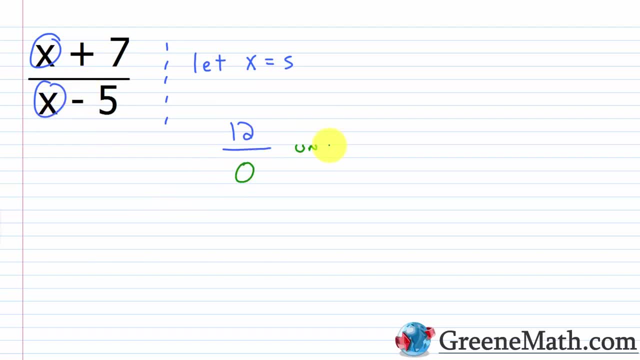 be 5 minus 5, which is, of course, 0, and again, this is undefined. Undefined, And this is what we're trying to prevent. We don't want to end up with something that's undefined. So what we do when we have a rational expression is we find our restricted value or our restricted values. 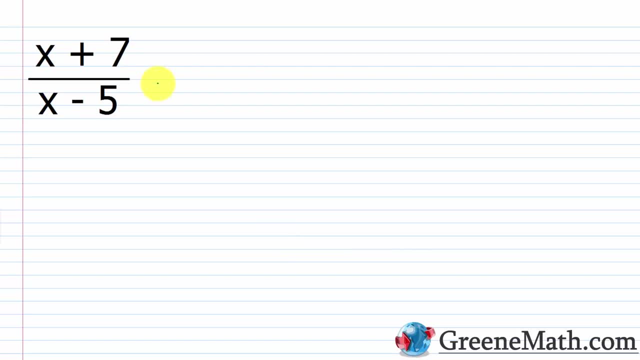 depending on how complex your rational expression is. and we just put a little note here. We say that this is defined for everything except for x when it's equal to 5.. So we'll put: x cannot be equal to, or x does not equal 5, okay. A fancier way to do this is to state the domain, okay, So 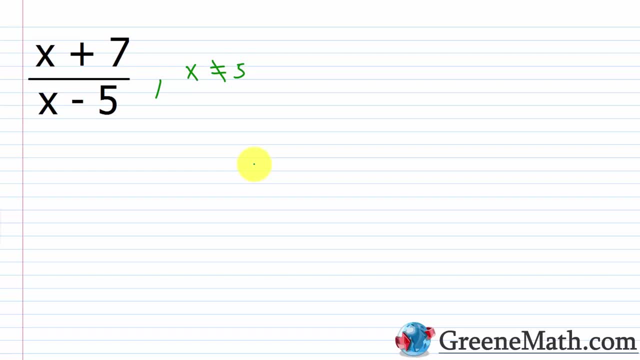 the domain. in case you haven't seen anything with functions yet- we'll talk more about this later in the course- the domain is the set of allowable x values. So what is allowed to be plugged in here for x? Well, everything in terms of the set of allowable x values is the set of allowable x values. 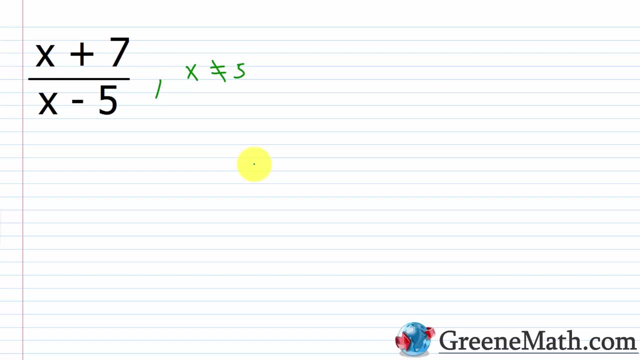 In terms of real numbers can be plugged in for x except for 5.. So the domain, or again the set of allowable values for x would say the set of all real numbers or the set of all elements x, such that x does not equal the number 5, okay. So anything you want to plug in for x, there is fine. 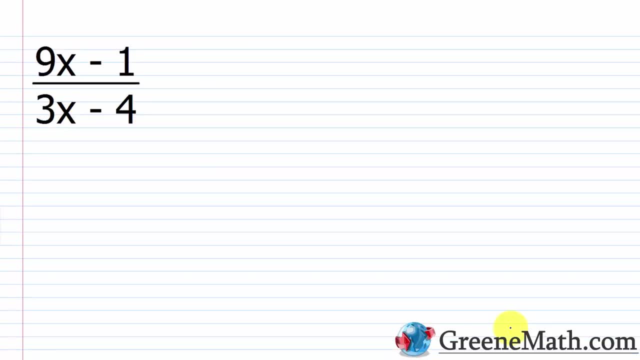 except for 5, because it makes the denominator 0.. All right, let's look at another example. So we have 9x minus 1 over 3x minus 4, again, all we need to do to find the restricted values. we take the denominator here and we just 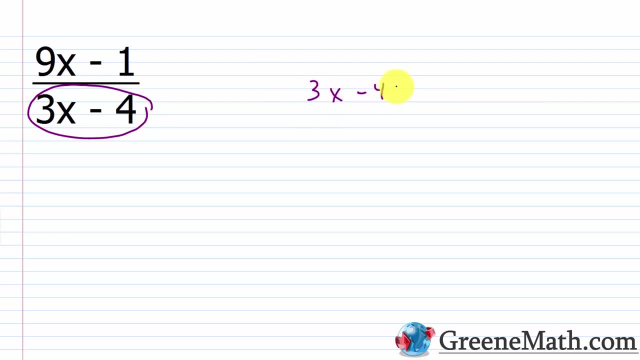 set it equal to 0.. So we're going to solve: 3x minus 4 equals 0.. To solve this, I add 4 to each side of the equation. that cancels. I would have 3x is equal to 4, divide both sides of the equation. 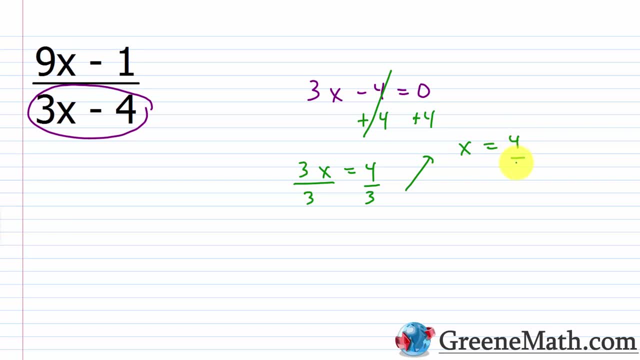 by 3, and I would end up with x is equal to 4 thirds. okay, So again I can write comma: x does not equal 4 thirds. Or I can do it in the fancy way, So I can say: my domain, okay, my domain. 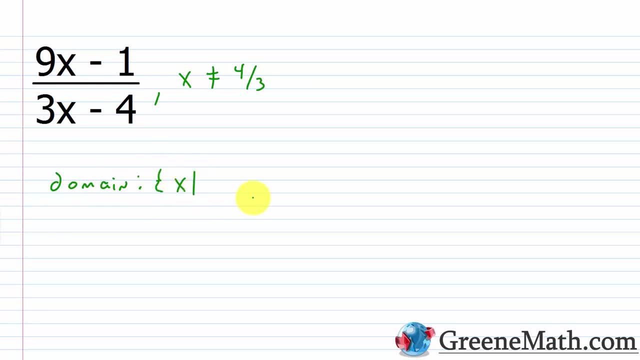 is the set of all elements, x, and then such that x does not equal 4 thirds. okay, All right, let's look at another one. So we have 2x squared plus 7x minus 4 over 3x squared minus. 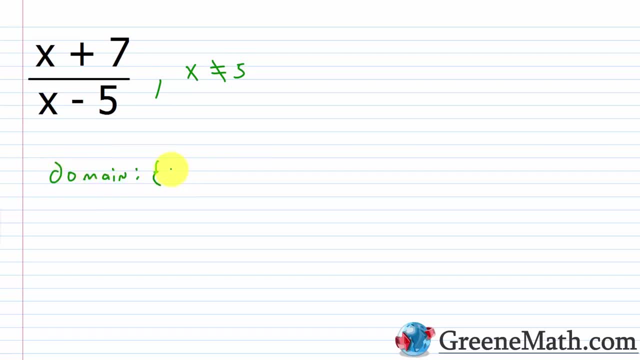 set of allowable values for X would say the set of all real numbers or the set of all elements, X, such that X does not equal the number 5. okay. so anything you want to plug in for X there is fine, except for 5, because it makes the 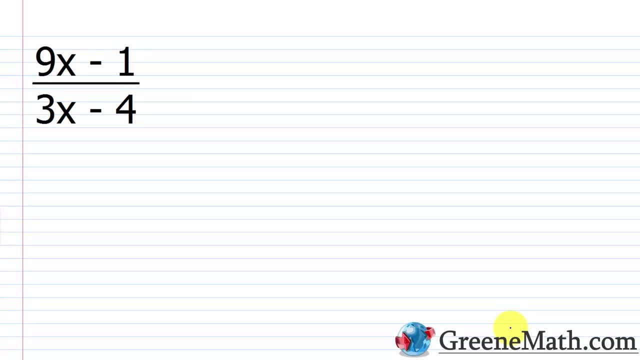 denominator 0. all right, let's look at another example. so we have 9 X minus 1 over 3 X minus 4. again, all we need to do to find the restricted values. we take the denominator here and we just set it equal to 0. so we're gonna solve 3 X minus. 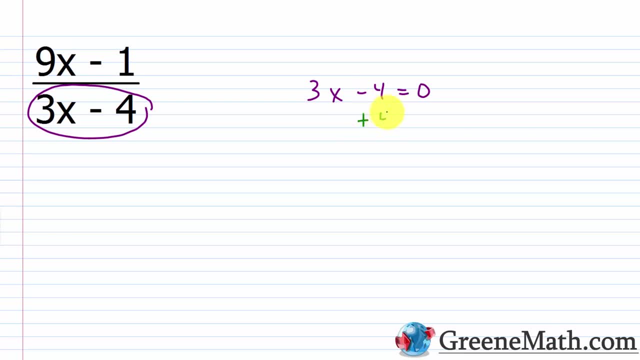 4 equals 0. to solve this, I add 4 to each side of the equation. that cancels. I would have 3. X is equal to 4. divide both sides of the equation by 3 and I would end up with X is equal to four thirds, okay. 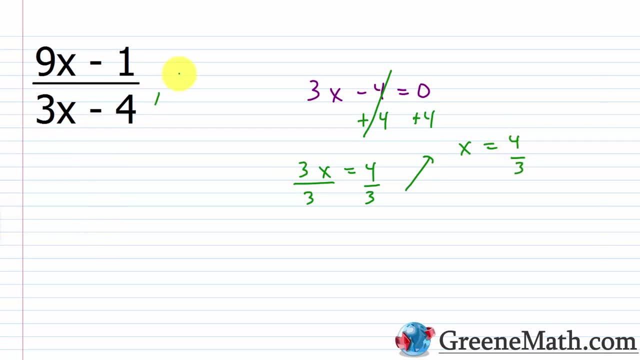 so again, I can write X not equal four thirds, or I can do it in the fancy way, so I can say my domain, and my domain is the set of all elements, X, and then such that X does not equal 4 thirds. okay, alright, let's look at another one. so we: 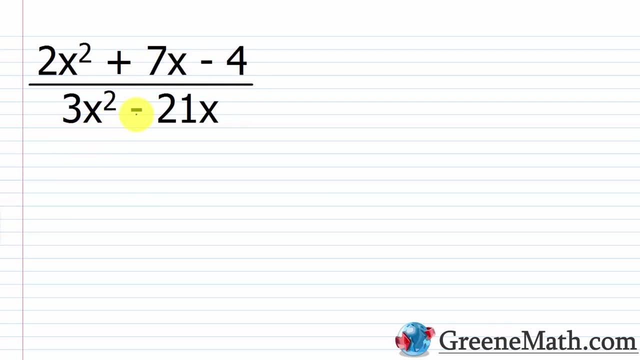 have 2 X squared plus 7 X minus 4, over 3 X squared minus 21 X. so again, I'm only concerned with the denominator here. So I'm just going to set this equal to zero and I'm going to solve it Now. you can get super complicated things in your denominator. 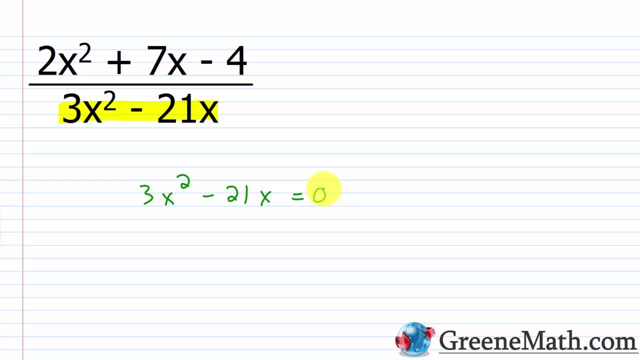 This guy right here is not complicated at all. We can solve it by factoring. In case you're not familiar with solving something by factoring, the first thing you would do is factor this guy. So we can see that we have a common factor of 3x. We can pull that out, So 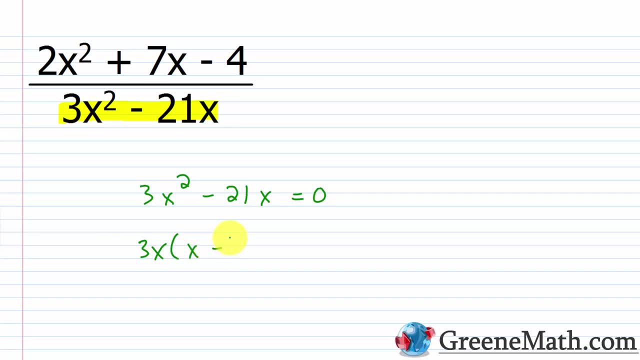 if we pulled out 3x, I would have an x minus 7 here, and this is equal to zero. Now what I'm going to do to solve this using factoring. I'm going to set each factor equal to zero, So I'm 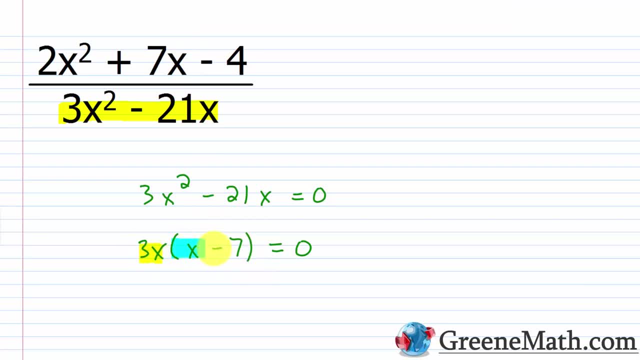 going to set 3x equal to zero, and I'm going to set x minus 7 equal to zero, and I'm going to solve each one of those. Now, why does that work? We have something known as the zero product property. So if you have something like a and it's multiplied by b and it's equal to zero. 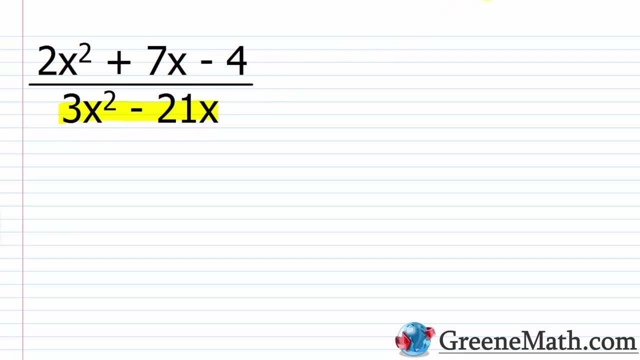 21x. So again, I'm only concerned with the denominator here, So I'm just going to set this equal to 0, and I'm going to solve it Now. you can get super complicated things in your denominator. This guy right here is not. 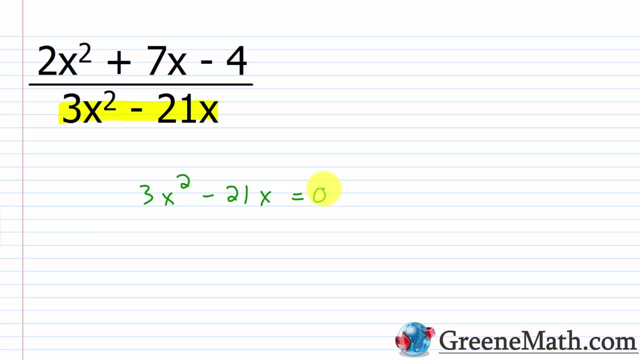 complicated at all. We can solve it by factoring. In case you're not familiar with solving something by factoring, the first thing you would do is factor this guy, So we can see that we have a common factor of 3x. We can pull that out. So if we pulled out 3x, I would have an x minus 7 here. 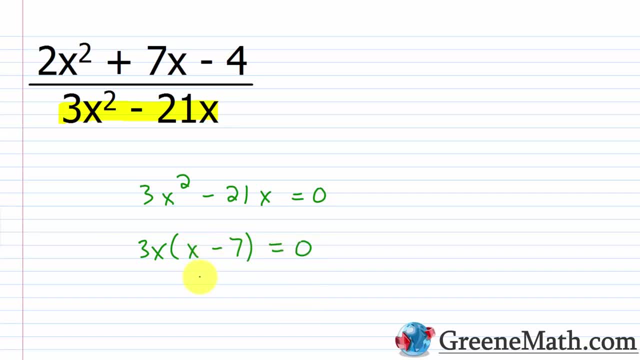 and this is equal to 0.. Now what I'm going to do to solve this using factoring. I'm going to set each factor equal to 0.. So I'm going to set 3x equal to 0, and I'm going to set x minus 7 equal to 0,. 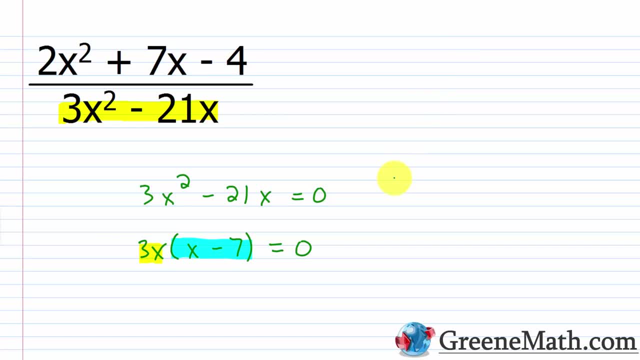 and I'm going to solve each one of those. Now, why does that work? We have something known as the zero product property. So if you have something like a and it's multiplied by b and it's equal to 0, well then, one of these statements has to be true. 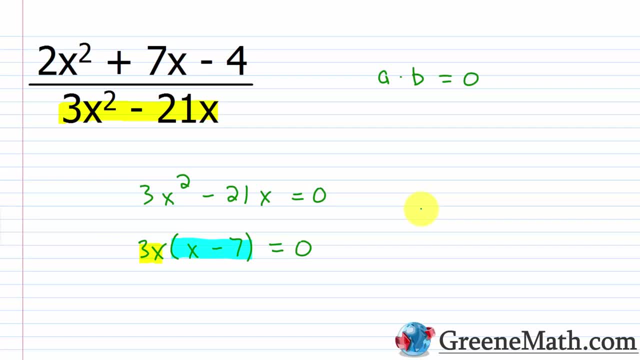 a is equal to 0, b is equal to 0, or both a and b are equal to 0. So, in other words, we know that multiplying by 0 gives me 0. So it could be true that a is 0 and b is not. It could. 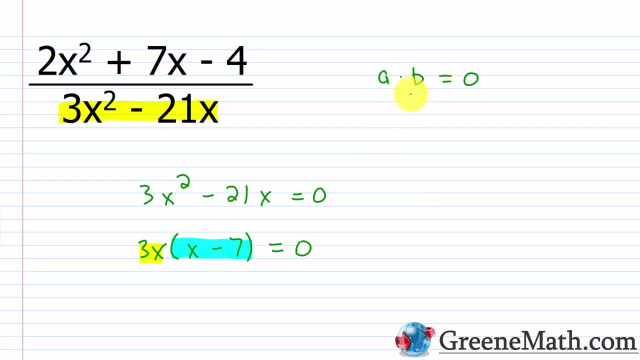 be true that b is 0 and a is not, and it could be true that a and b are both 0.. So that's the premise behind the zero product property, and essentially all I'm going to do here is just set 3x equal to 0 and solve, Divide both sides by 3.. I get x is equal to 0. I'm going to set x minus 7. 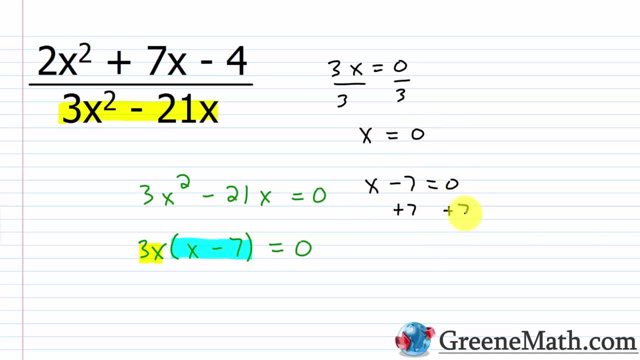 equal to 0 and solve, Add 7 to each side of the equation. I get x is equal to 7.. So we have two solutions here and thus two values we need to restrict from our domain. So if I plugged in a 7 for x or if I plugged in a 0 for x, I would get 0 as a denominator. 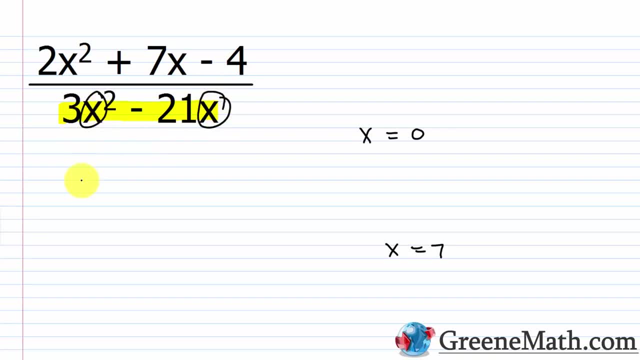 And I think we can see that right. If you plugged in a 0 here and here, you would have 3 times 0 squared minus 21 times 0.. 0 squared is of course, 0.. 0 times 3 is 0,. 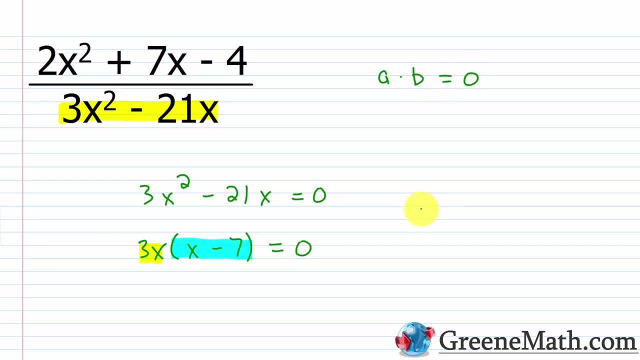 well then, one of these statements has to be true: A is equal to zero, b is equal to zero, or both a and b are equal to zero. So, in other words, we know that multiplying by zero gives me zero. So it could be true that a is zero and b is not. It could be true that b is zero and a is. 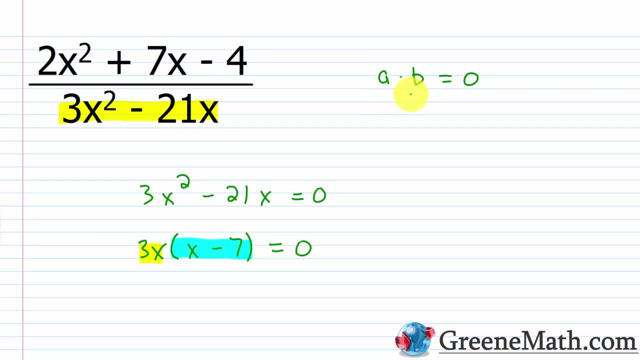 not, And it could be true that a and b are both zero. So that's the premise behind the zero product property, And essentially all I'm going to do here is just set 3x equal to zero and solve, Divide both sides by 3, I get x is equal to zero. I'm going to set x minus 7 equal to zero. 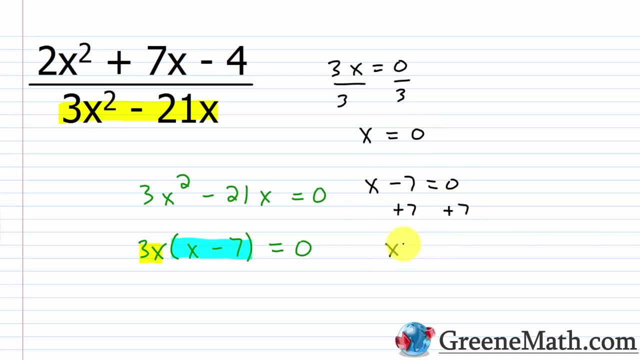 and solve: Add 7 to each side of the equation I get x is equal to 7.. So we have two solutions here and thus two values we need to restrict from our domain. So if I plugged in a 7 for x, or if I 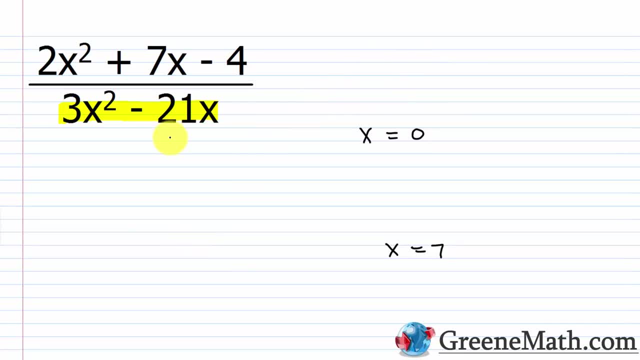 plugged in a zero for x, I would get zero as a denominator, And I think we can see that right. If you plugged in a zero here and here, you would have three times zero squared minus 20, 21 times zero. Zero squared is of course, zero. Zero times three is zero Minus zero times 21 is. 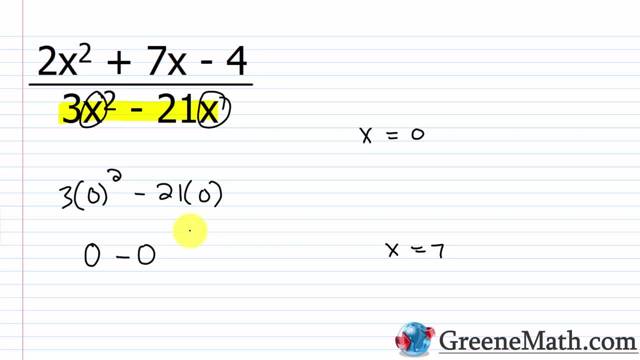 zero. Zero minus zero is zero, So the denominator would be zero. if you plugged in a zero for x. Okay, so we see that Also, the denominator would be zero if you plugged in a seven. Seven squared is 49.. 49 times three is 147.. So you'd have 147 minus 21 times seven is also 147.. 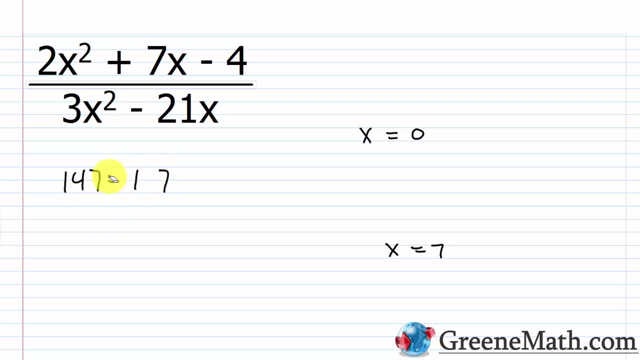 So you get 147 minus 147, which is zero. So we're going to write that x cannot be zero and x cannot be seven. Let me kind of scooch these up. I'll scooch this up, So I'll put a comma here and you can put a comma there if you want. So again, 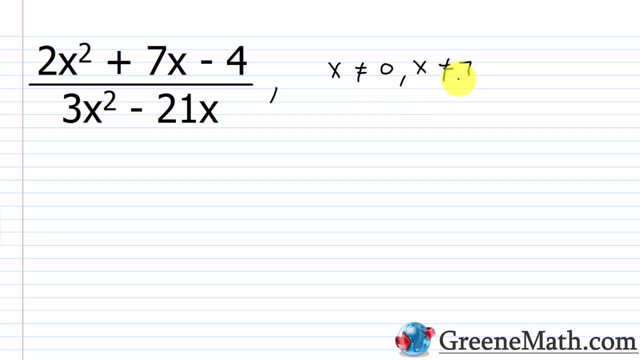 all real numbers are allowed except for zero and seven. So we can write this again in this kind of fancy way: The domain is the set of all elements, x, such that x does not equal zero or seven. All right, let's take a look at one more. So very easy concept overall, The only thing that can make. 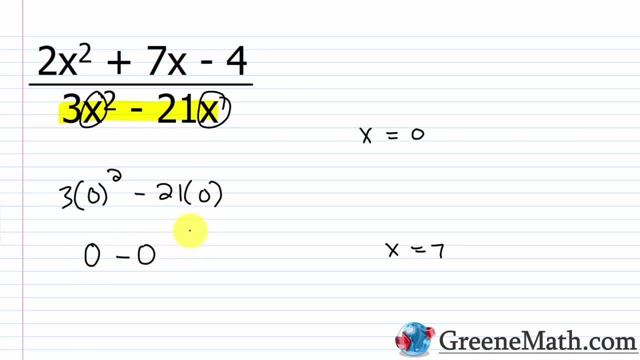 minus 0 times 21.. 0 minus 0 is 0.. So the denominator would be 0 if you plugged in a 0 for x. Okay, so we see that Also, the denominator would be 0 if you plugged in a 7.. 7 squared is 49.. 49 times 3 is 147.. 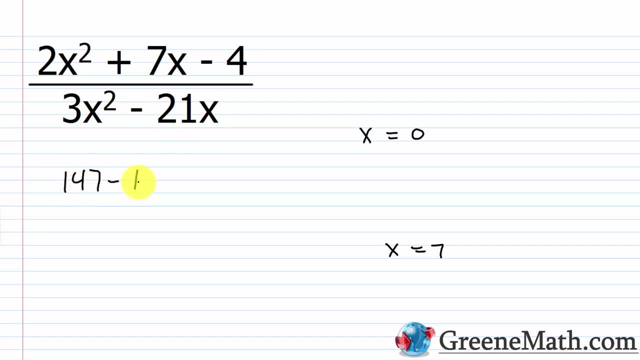 So you'd have 147 minus 21 times 7 is also 147. So you get 147 minus 147, which is 0.. So we're going to write that x cannot be 0 and x cannot be 7.. Let me kind of scooch these up. 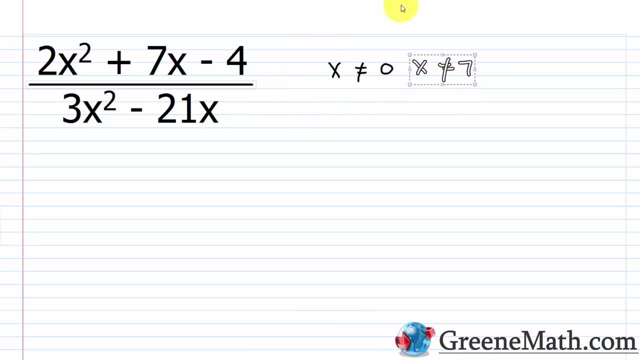 I'll scooch this up. So I'll put a comma here and you can put a comma there if you want. So again, all real numbers are allowed except for 0 and 7. So we can write this again in this kind: 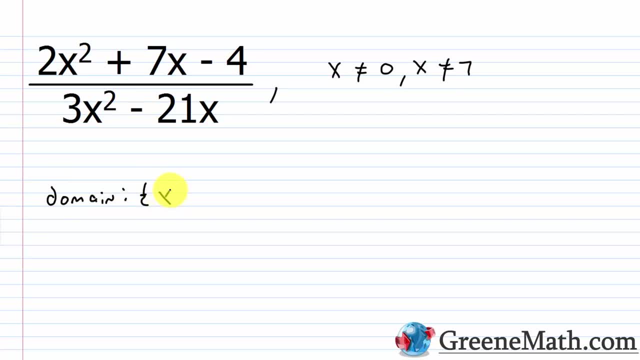 of fancy way, The domain is the set of all elements, x, such that x does not equal 0 or 7.. All right, let's take a look at one more. So very easy concept overall, The only thing that can make it more difficult. 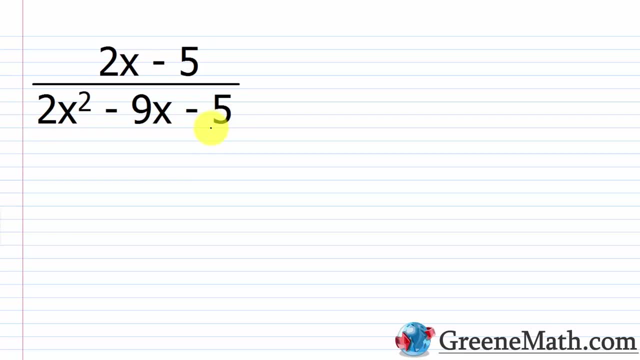 is the tediousness of the denominator right? If you get something that's super complex, it might not be so easy to solve. You can't solve everything with factoring. You might have a very, very difficult denominator to work with, But for this, 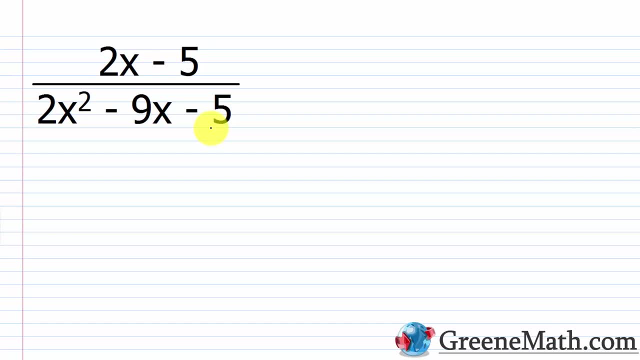 I'm just trying to show you the concept, So I gave you things that are pretty easy. So we have 2x minus 5 over 2x squared minus 9x minus 5.. I'm just going to set again. 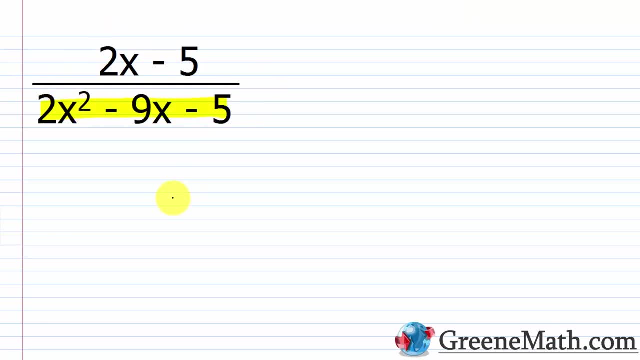 this guy right here- equal to 0.. So 2x squared minus 9x minus 5.. 9x minus 5 equals 0. So here we're not going to factor out the greatest common factor, We're going to factor this into the product of two binomials. So I'm going to do this using 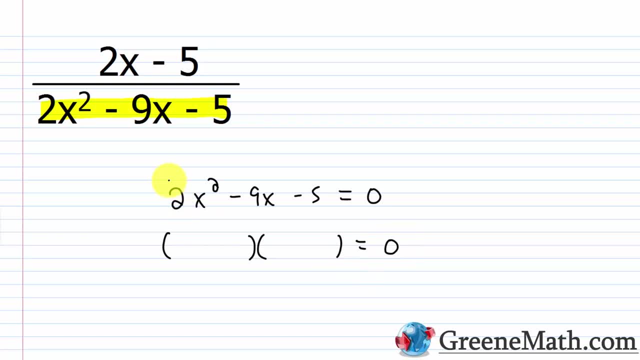 reverse FOIL. And the reason I'm going to choose reverse FOIL is because this coefficient here- this 2, is a prime number. So I know this would be 2x and this would be x. I just have to work out the correct outer and inner right. So I know that I want a product of negative 5. So that can. 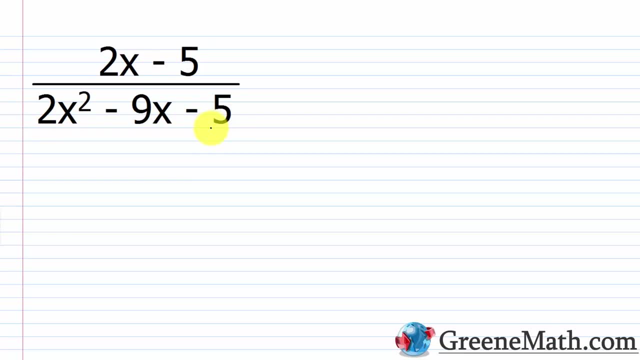 it more difficult is the tediousness of the denominator. right, If you get something that's super complex, it might not be so easy to solve. You can't solve everything with factoring. You might have a very, very difficult denominator to work with. But for this, 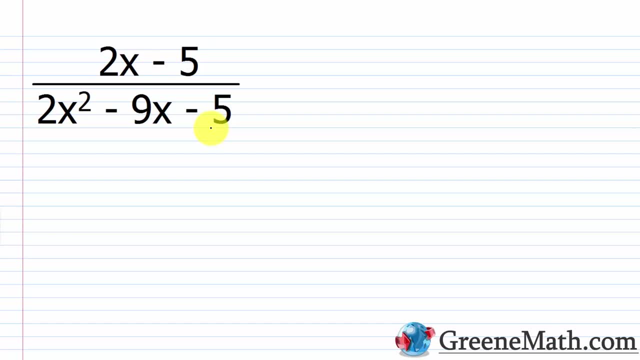 I'm just trying to show you the concept, So I gave you things that are pretty easy. So we have two x minus five over two x squared minus nine x minus five. I'm just going to set again this guy right here equal to zero. So two x squared minus nine x minus five equals zero. 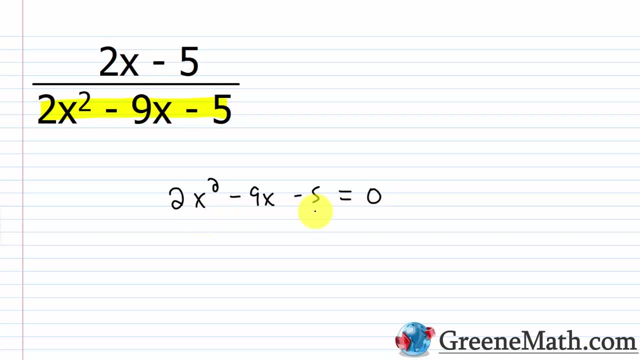 So here we're not going to factor out the greatest common factor, We're going to factor this into the product of two binomials. So I'm going to do this using reverse FOIL. The reason I'm going to choose reverse FOIL is because this coefficient, here, this two, is a prime number. So I know this would. 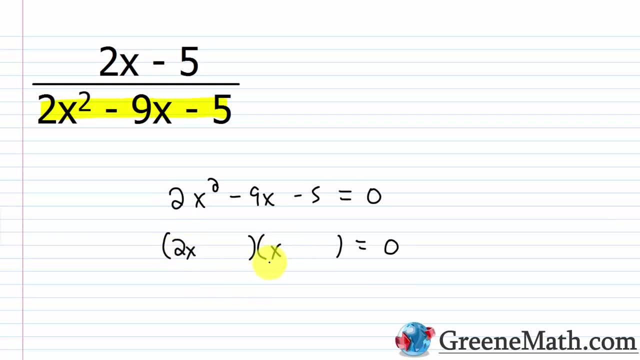 be two x and this would be x. I just have to work out the correct outer and inner right. So I know that I want a product of negative five. So that can only come from five times one, with the signs being different right. So I got to have either negative one times five or negative five times one. 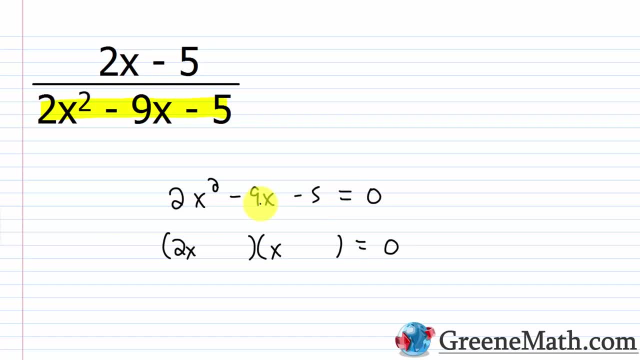 So, knowing that I have a middle term of negative nine x, I'm going to want to multiply two x by negative five And I'm going to multiply x by positive one. right, Two x times negative five would give me negative 10 x, And then one times x would give me. 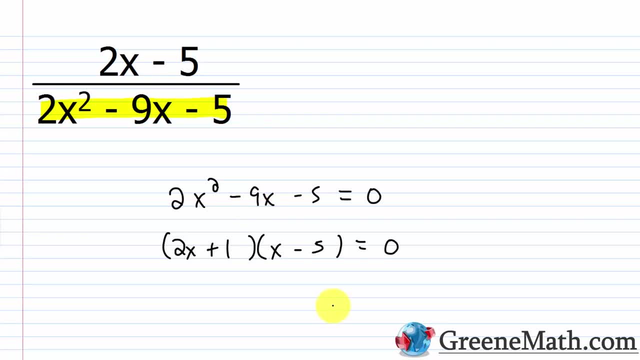 one x. one x plus negative 10 x would be negative nine x. So we factored this one pretty quickly, All right. So now I'm just going to set each factor. This is a factor, and this is a factor equal to zero. So I would have two x plus one equal to zero, and I would have x minus five equal. 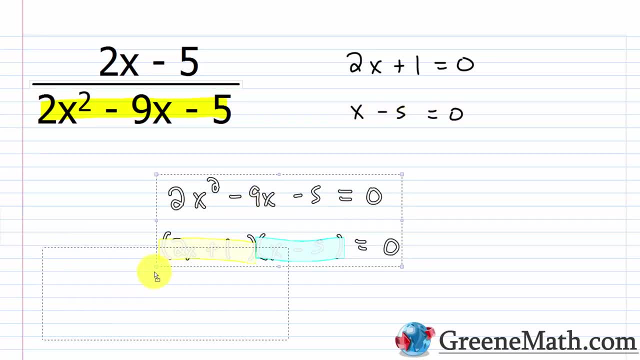 to zero. So let me kind of slide this out of the way so we have a little room. So for this guy, let me kind of scooch this down. For this guy, I'm going to subtract one away to start. So this cancels. I would have two. x is.